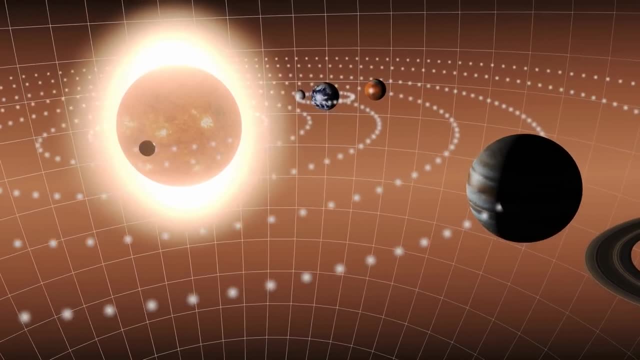 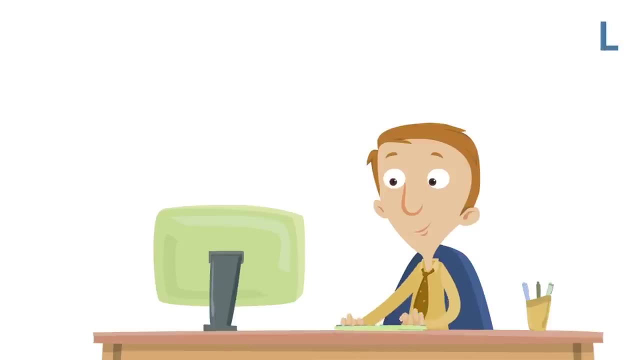 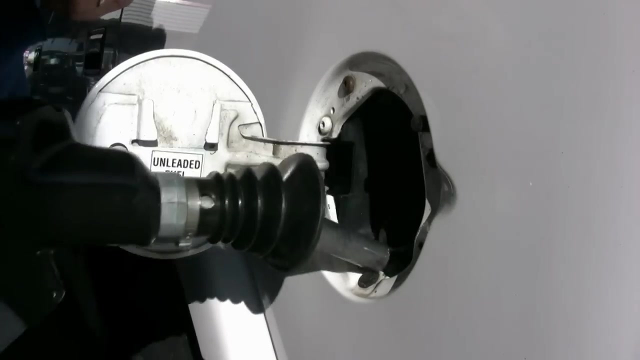 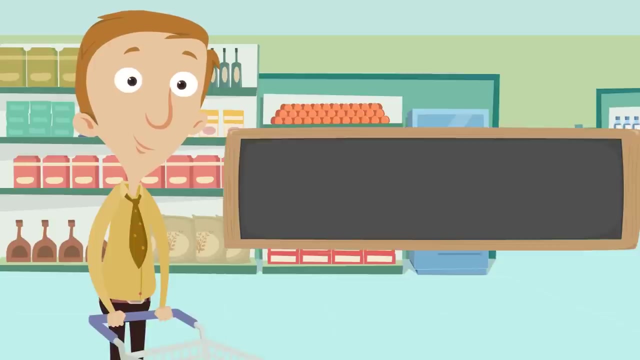 center of our solar system, But the sun really is a regular star, Like other stars, the sun uses hydrogen to burn bright. Hydrogen is the sun's fuel, just like food is our fuel and gasoline is the fuel, The sun uses hydrogen as fuel. If you're wondering what hydrogen is, hydrogen is a gas found all over. 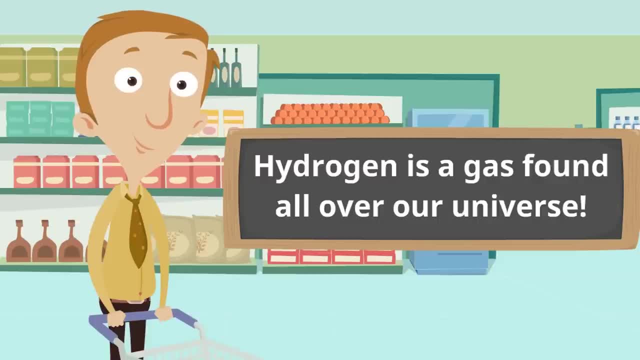 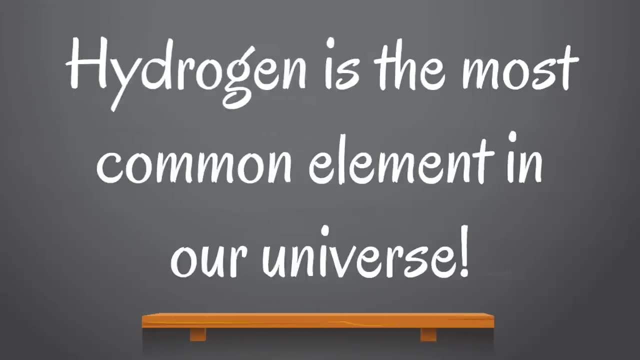 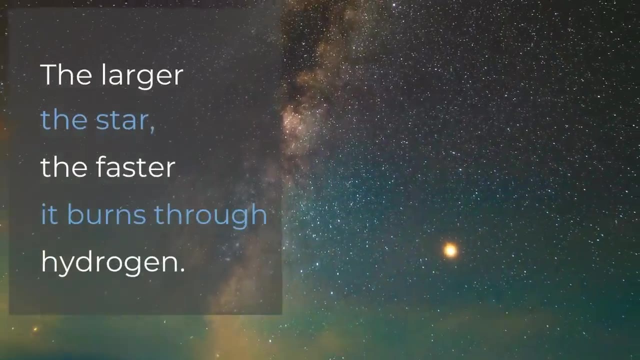 our universe, And it's hard to see because it doesn't have any color to it, But it's all over the place. In fact, hydrogen is the most common element in our universe, So stars use a gas called hydrogen as fuel. The larger the star, the faster it burns through hydrogen. 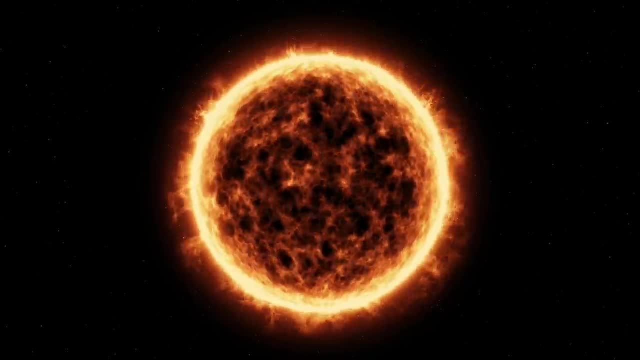 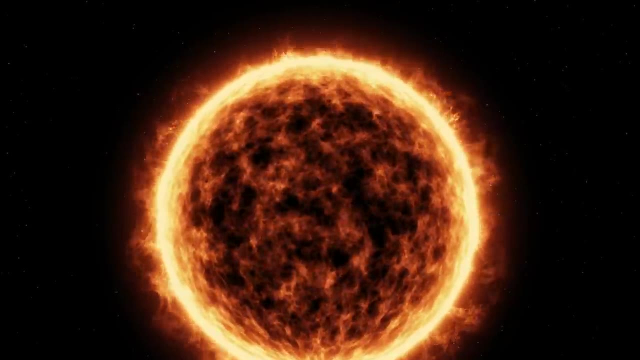 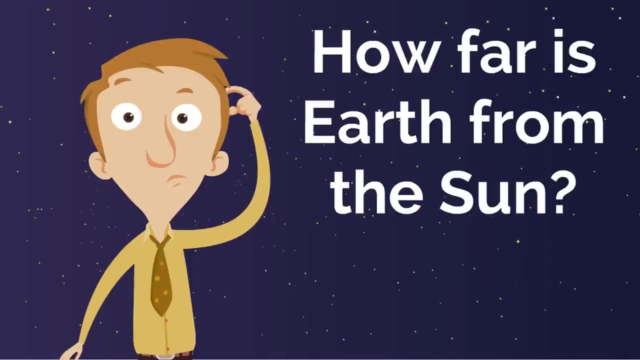 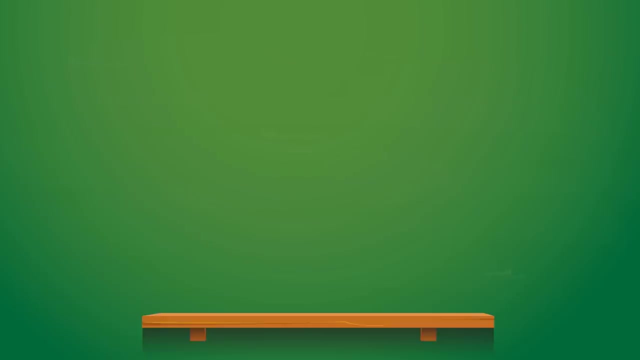 Thankfully, the sun has at least a 5 billion year supply of hydrogen left, so the sun will keep burning for a long time. Here's an interesting question: How far is Earth from the sun, How far is our planet from this huge star in the center of our solar system? Well, it's pretty far away. It's pretty far away The sun is. 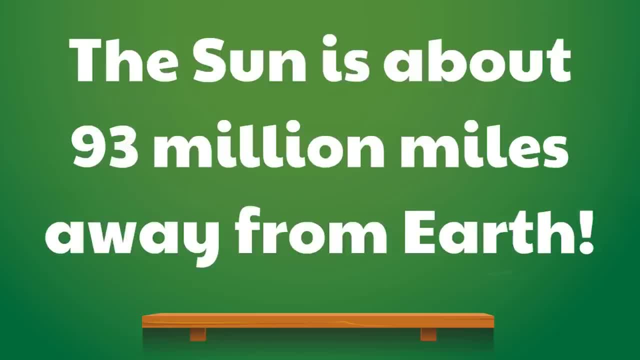 about 93 million miles from our solar system. Well, it's about 93 million miles from our solar system. Well, it's pretty far away. It's pretty far away. The sun is about 93 million miles from our solar, away from Earth, That's right, about 93 million miles away from our planet Earth. 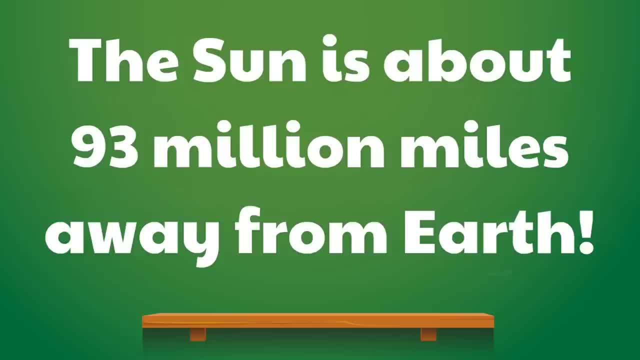 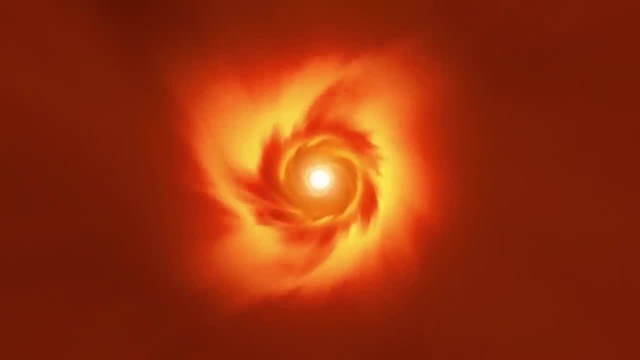 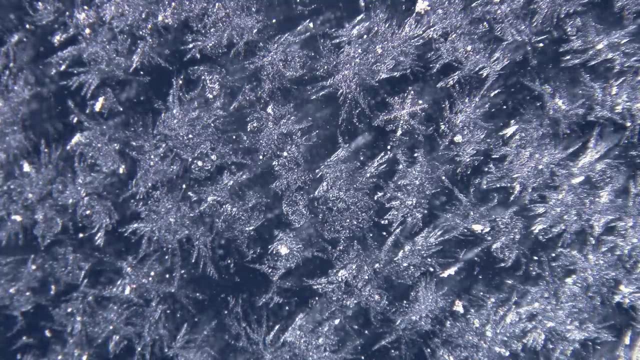 And it's a good thing. It's a great thing that the sun is about 93 million miles away, because if we were any closer to the sun it would be way too hot to sustain life, And if we were further away we would all freeze. It would be way too cold. So the sun is the 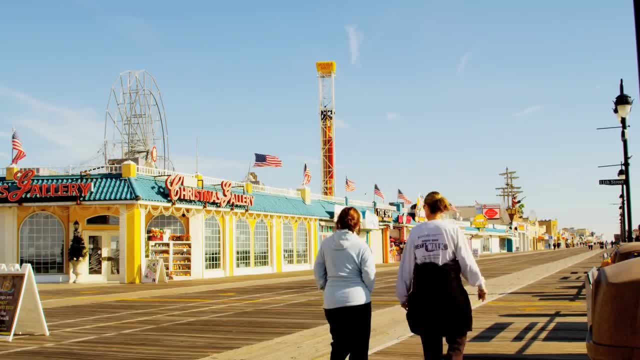 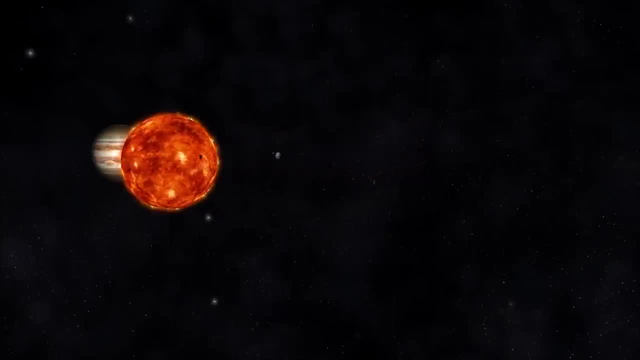 perfect distance away from the Earth. Of course, having a huge star 93 million miles away helps us to see things right. It is helpful to have a massive burning light in the middle of our solar system that runs on hydrogen. I mean, can you imagine living in a world without light? 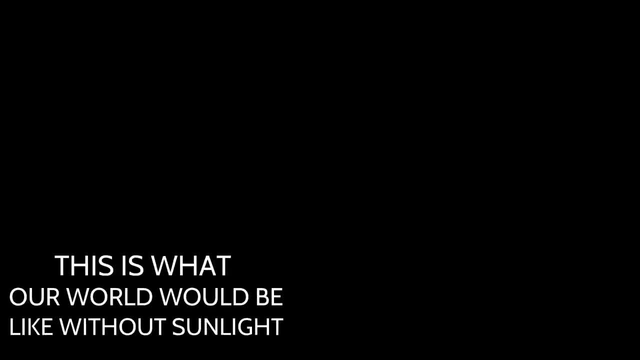 It would be like this: This is what our world would be like without sunlight: It would just be dark. You know, we wouldn't be able to see anything. We'd be like bumping into each other and it'd be crazy. We'd be like: oh wow, is that a mountain or is that a chicken, or 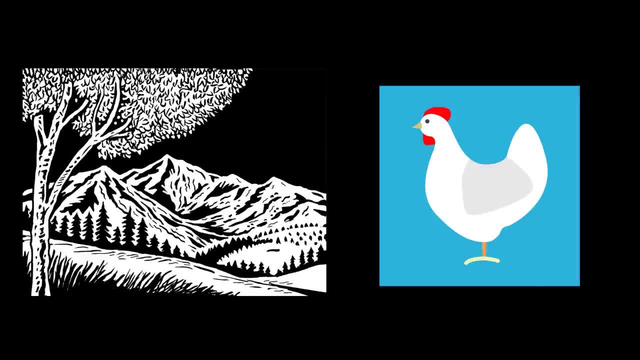 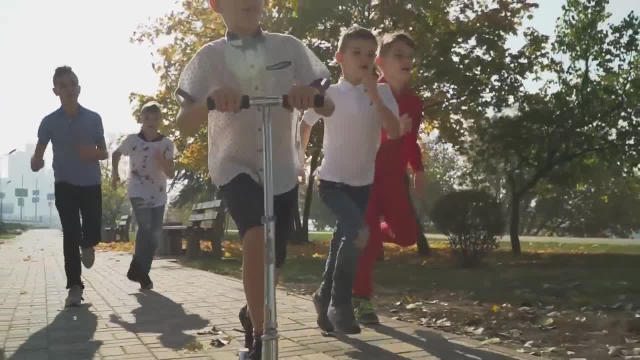 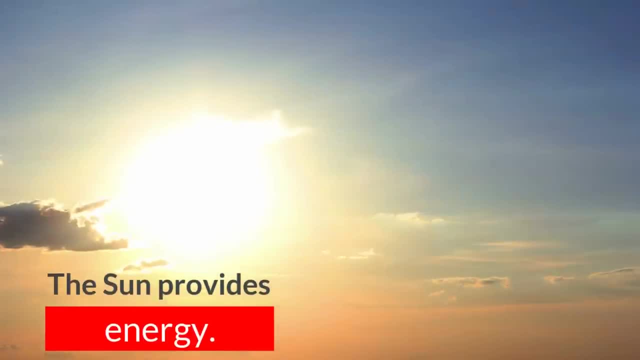 what's going on? Where am I? What's going on? The sunlight allows our eyes to see what's going on around us, But the sun provides more than just sunlight: The sun provides energy. One powerful way the sun provides energy is through a process called photosynthesis. Wow, that's a big word, Can? 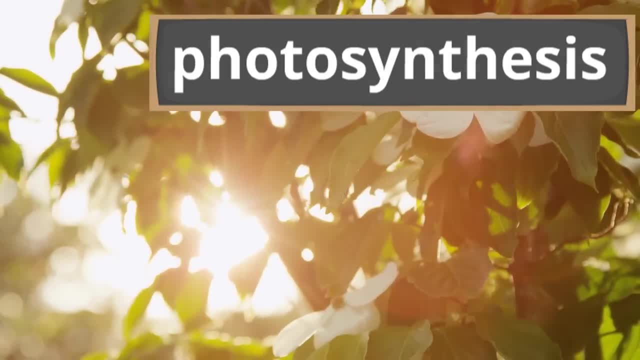 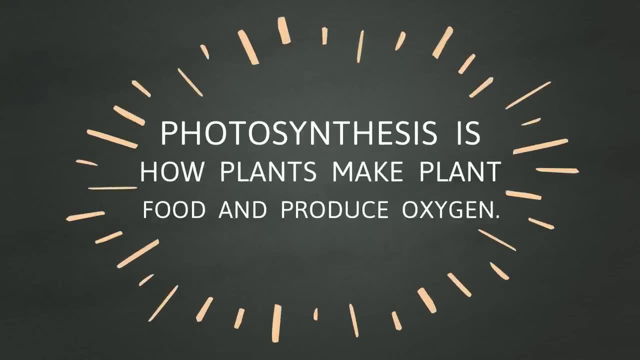 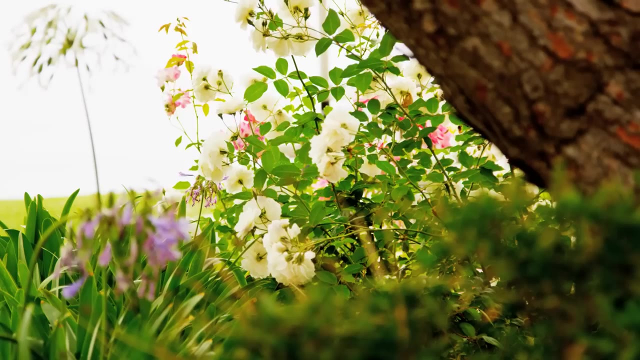 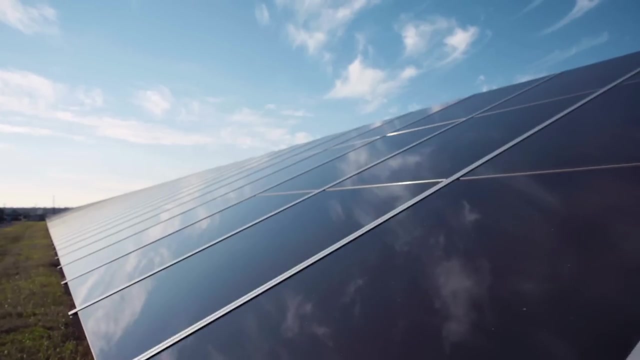 you say that Photosynthesis, Yeah, photosynthesis. Photosynthesis is how plants make plant food and produce oxygen. Without sunlight, plants cannot make plant food or release oxygen. You know, plants are not alone in using sunlight for energy. We use sunlight for energy as well. 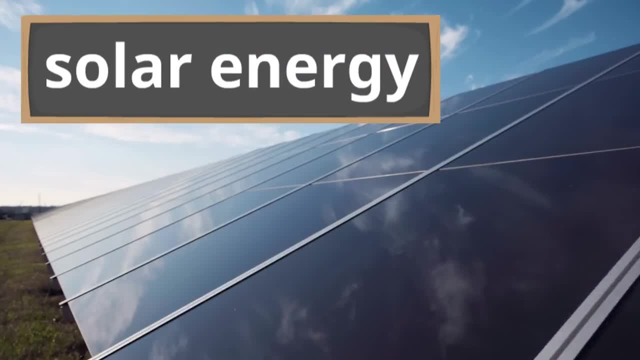 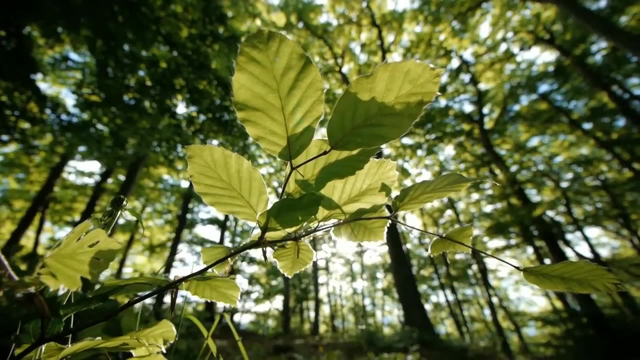 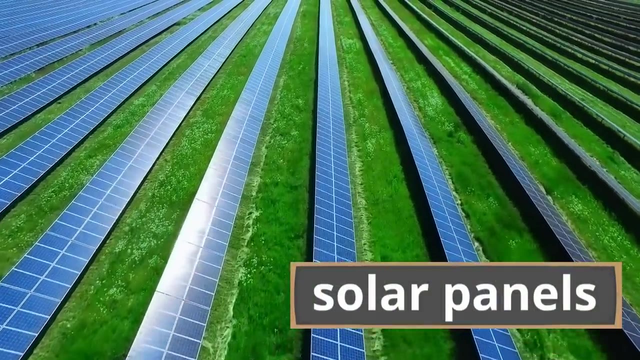 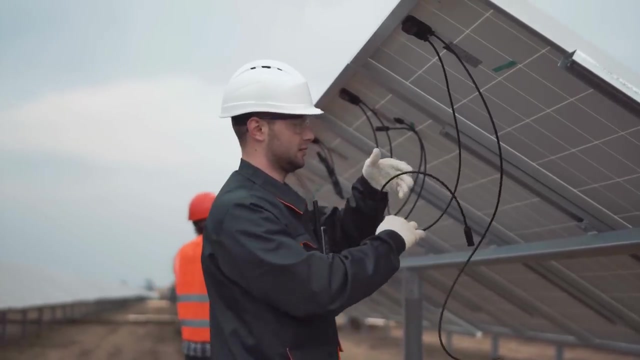 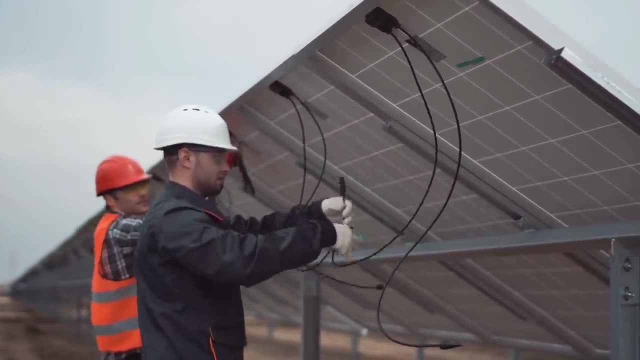 The energy we get from sunlight is called solar energy. Just like plants capture sunlight in the process of photosynthesis, people capture sunlight using these things called solar panels. Isn't that cool. Here are two men installing solar panels. The sun is powerful. It is awesome to see how we can use some of its energy to get power and electricity. 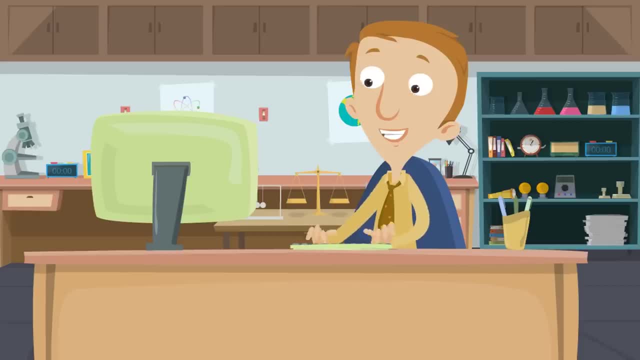 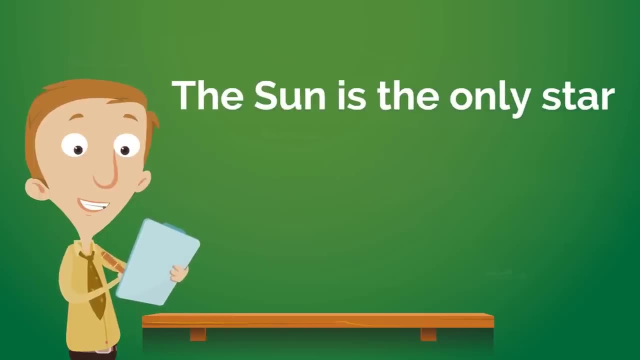 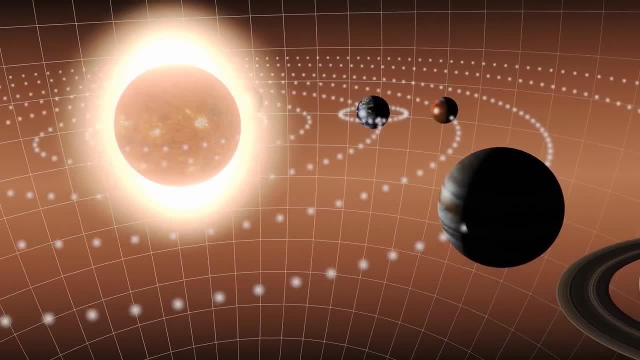 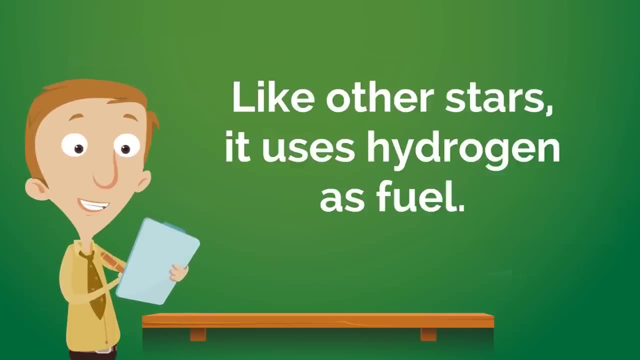 Uh-huh, right in the middle. Yeah, Like other stars, it uses hydrogen as fuel. Thankfully, it has a lot of hydrogen, so it will keep burning and burning for a long time. Isn't that cool? Isn't that cool? It has a lot of hydrogen, so it will keep burning and burning for a long time. Yeah, it is cool. It shares energy with other stars too. It has an incrediblegirl strength. Yeah, Let's talk about reg pants after theanto. 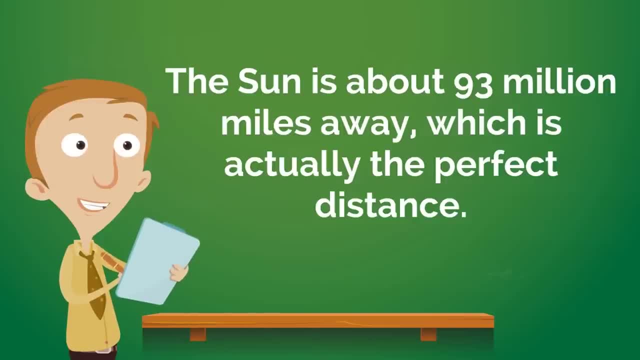 We learned that the sun is about 93 million miles away, which is actually the perfect distance. If the sun were further away, it would be too cold. if it was closer, this planet would be way it would be too cold. if it was closer, this planet would be way too hot. 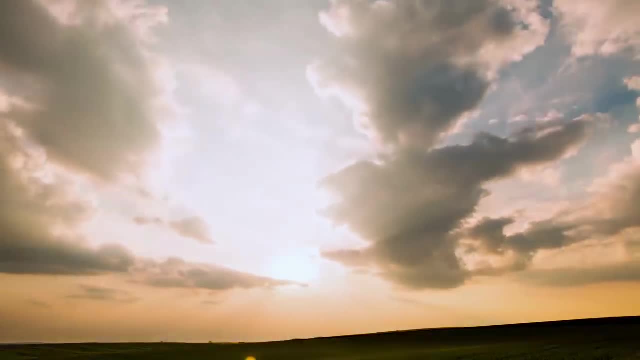 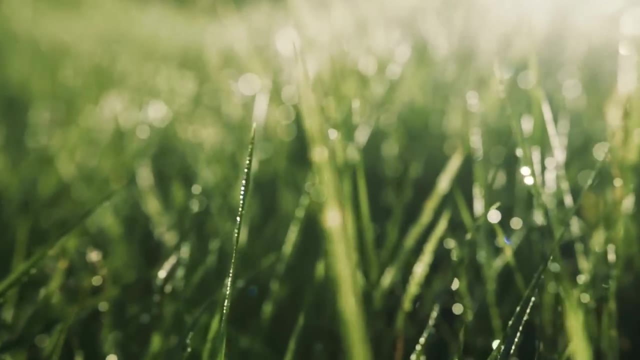 too hot. We also learned that the sun not only provides light, it brings energy. We also learned that the sun not only provides light, it brings energy. Plants use energy from the sun in a process called photosynthesis, and people get energy from the sun using things like solar panels.